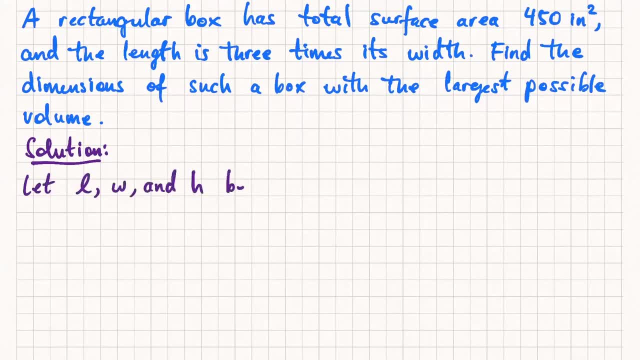 let L, W and H be the length, height and the width of the box We want to maximize. So Caleb told me the objective function is a function of three variables- L, W and H- And it's just the product of those three. So that's the objective function. 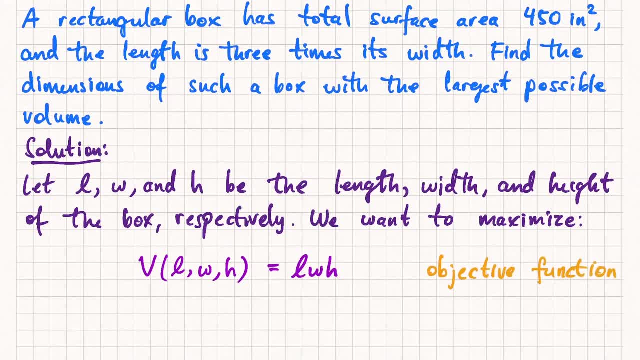 This is the thing that we are eventually taking the derivative of. The only problem is we have three variables. So we're going to take the derivative of L, W and H and it's just the variable. So we're going to take the derivative of L, W and H and it's just the product of three. 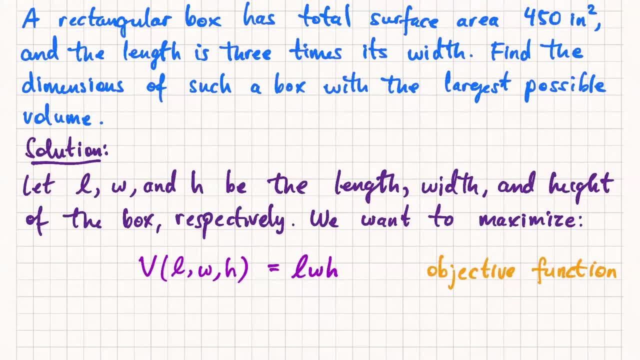 variables. Harsh- Uh-oh, Harsh didn't think I'd call on him. If we have three variables, how many constraints do you think we need? And I think we need three. You think you need three? Well, in the previous examples we had two variables. 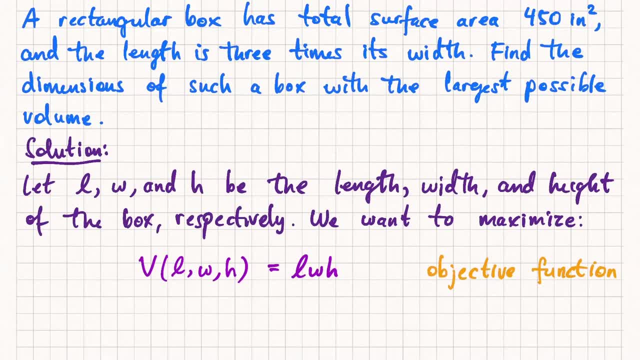 And so one constraint got it down to one variable. So in this case, if I have three variables, how many do we need? We actually need two constraints. Each constraint eliminates one variable, So you need two constraints, And so we have three variables, And so we have three. 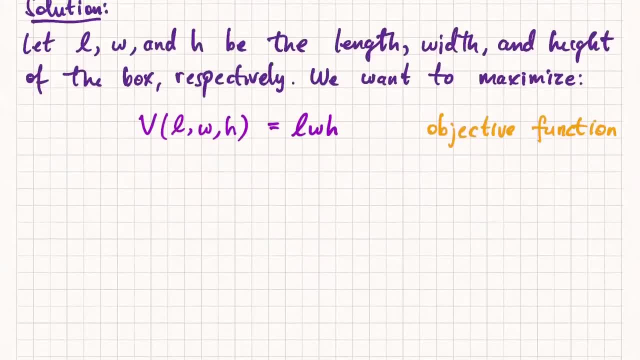 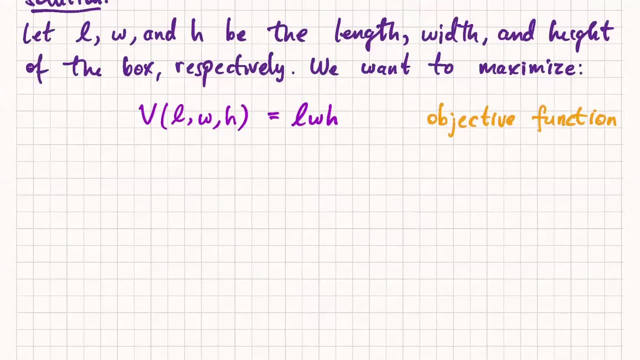 constraints, And so we have three variables, And so we have three constraints. And so we have two constraints in this problem. Okay, Because I think two variables- it's kind of like flawed logic, but two variables equals one. Well, the idea is one constraint. So for instance in the previous problem, H equals 2,000 over R. 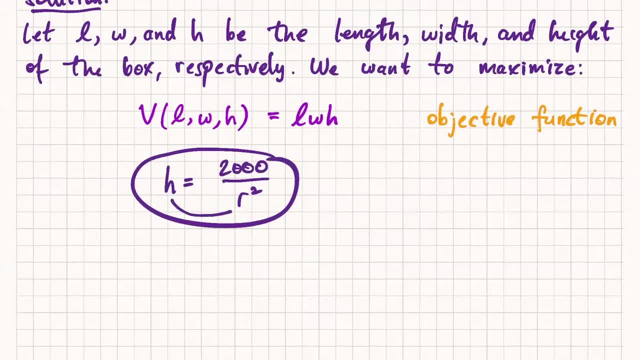 squared. So one constraint gives you one variable in terms of the others. That eliminates H from the objective. So each constraint eliminates one variable. So if I have three and I'm going to get down to one, I need two constraints, Okay. 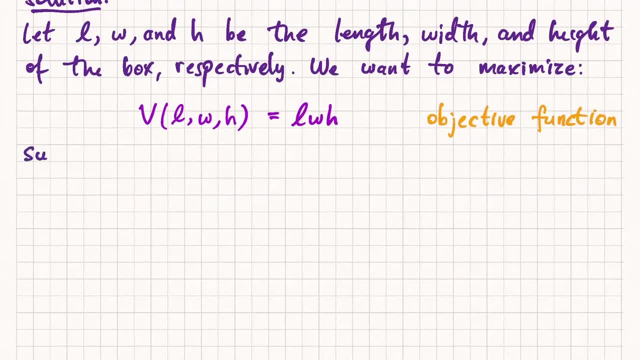 Okay, Okay. So we want to maximize this subject to the constraints, Subject to the two constraints. And someone says now you use: L equals 3W. LOL, That is correct, L mal. So one constraint is going to be L equals 3W. 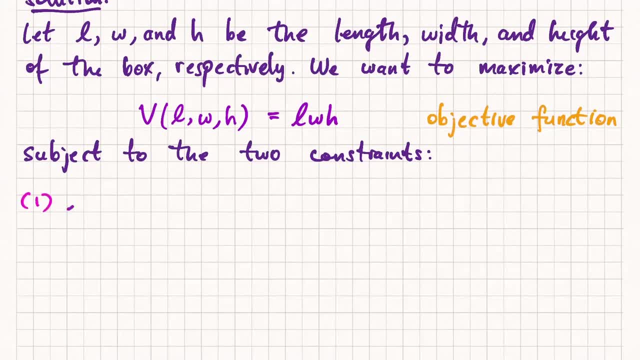 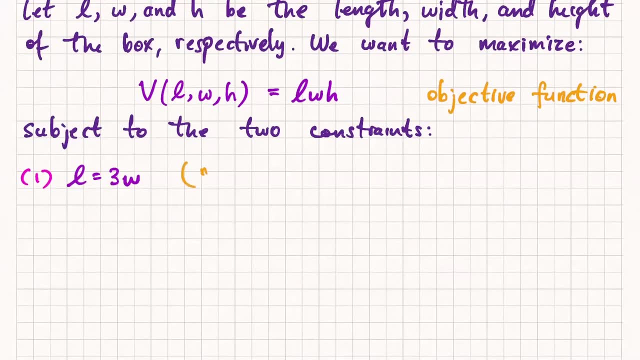 Was that actually it? Yeah, the length is three times Yeah. So the problem said length is three times width. So that is one constraint. Now I need another constraint. What is going to be the second constraint of my problem? Let me zoom out a little bit. You don't necessarily have to give. 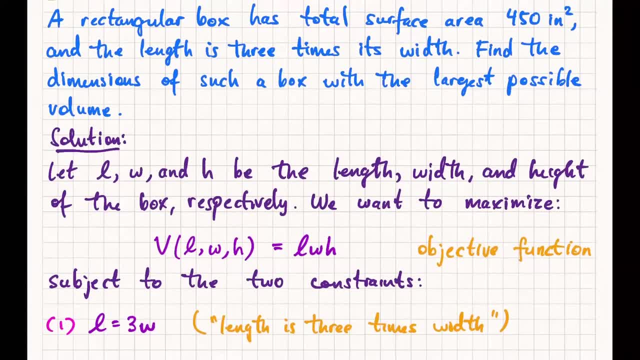 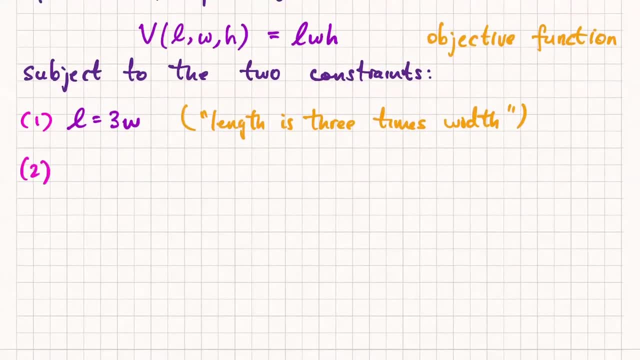 me a full equation. Okay, good. So Jacqueline says 450 has to equal the surface area, Right, Okay, Uh huh, Okay. So you say: can you also dim the surface area? Okay, Okay. So let's put that down over here. 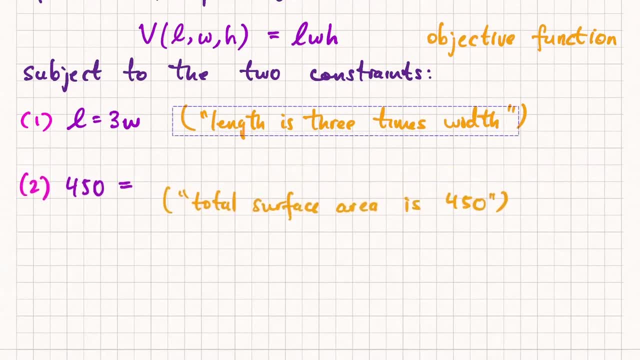 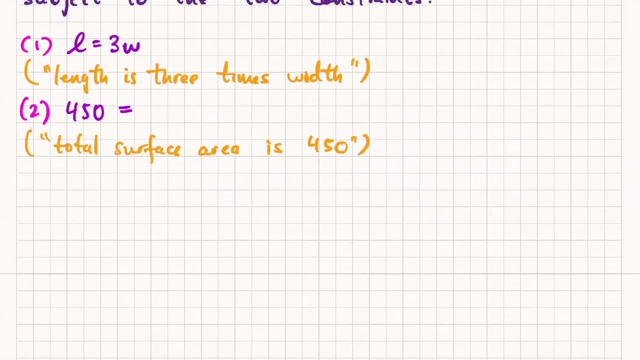 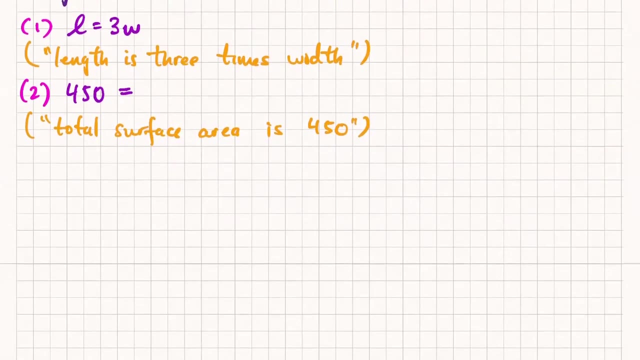 And we can go ahead and activate this. Wow. so what is this equation? what is the total surface area of this box? do we need a diagram? i think we're going to need a diagram: l1, w1, l2, w2, i don't know what. there's only one l. why are we getting l1 and l2? what does this mean? 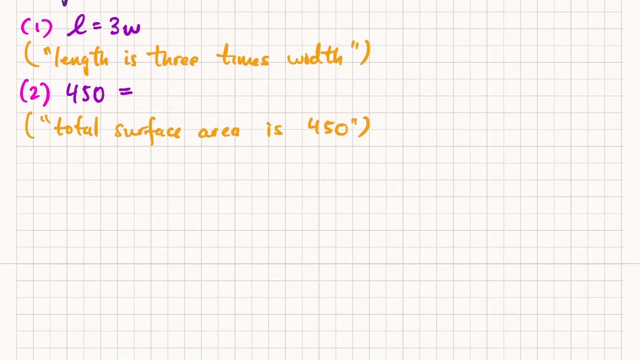 why we got what we got so many widths. okay, so let me, let me draw an ugly box, then i'll make it nice later. hold on, actually, wait a second. i have a good box there, it is. yeah. there you go. that's a. that's a diagram of a box. so how many faces? 450 equals 6x squared. so first, 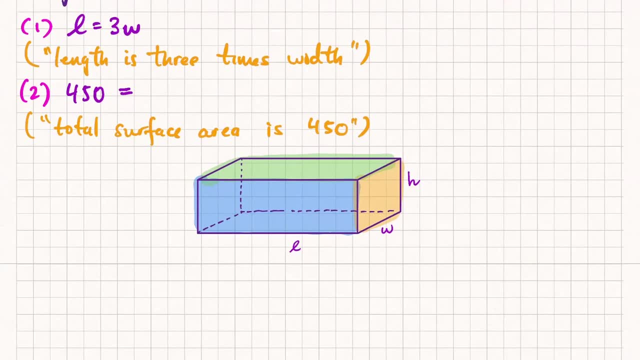 of all, we don't, we're not using the variable x and 456 x squared. i want to be very clear. how can you tell right away that this is absolutely not the constraint, because it's not giving you one variable in terms of the other? If you thought, 450 equals 6x squared. 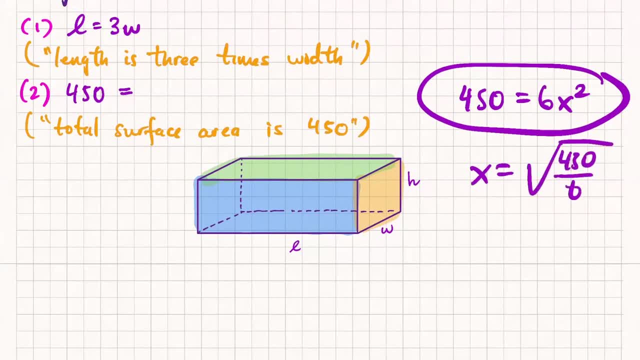 you can just say: x equals square root 450 over 6.. And now you suddenly have: yeah, I mean, it's not a cube, But if you have an equation involving only one variable, that's not a constraint. That's literally telling you what. 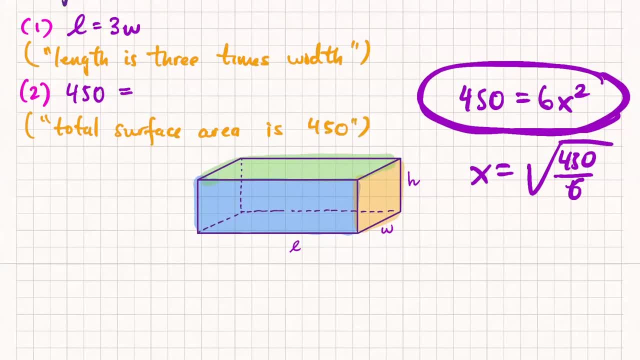 the dimension of the box is: And there's no problem anymore. There's no find the box of largest volume because there's only one box. Only one box can satisfy this equation. So make sure you account for all six faces. There's six faces to a box. 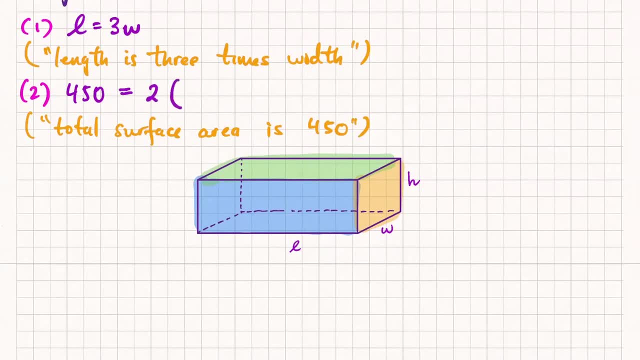 And so 450 has to equal 2.. So they come in pairs, three pairs, So I think Margaret has it. So Lw plus Lh plus Wh, And multiply the whole thing by 2. And that has to equal 450.. 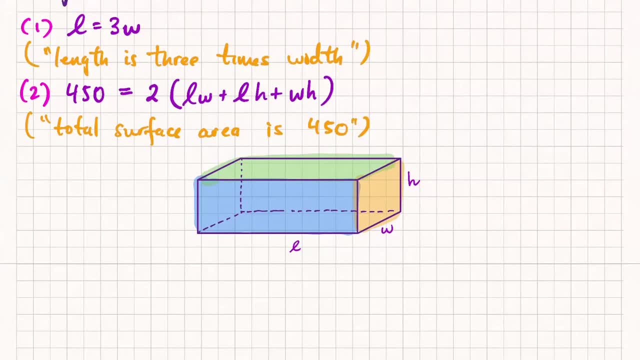 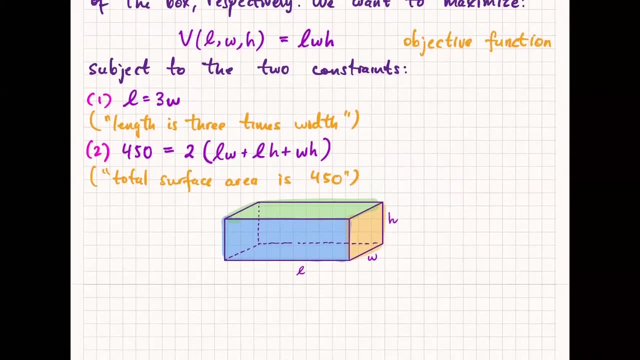 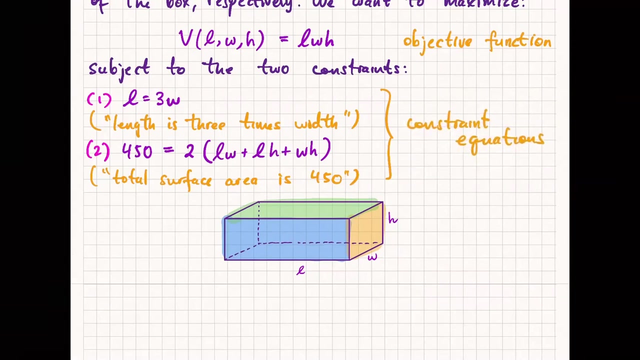 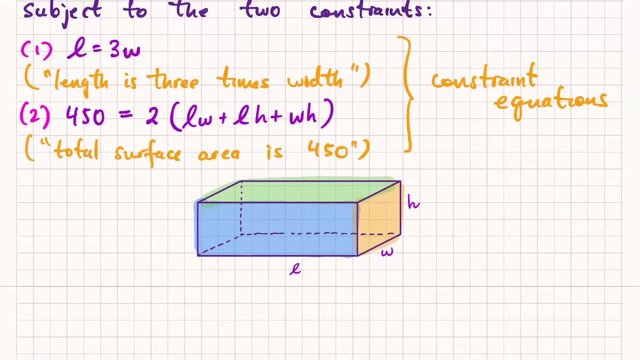 Good, OK, now we have to do what. What is the next goal in our problem? Identify the objective, And I identified my two constraints. What would be the next goal of the problem? Solve with respect to W for constraint 2.. 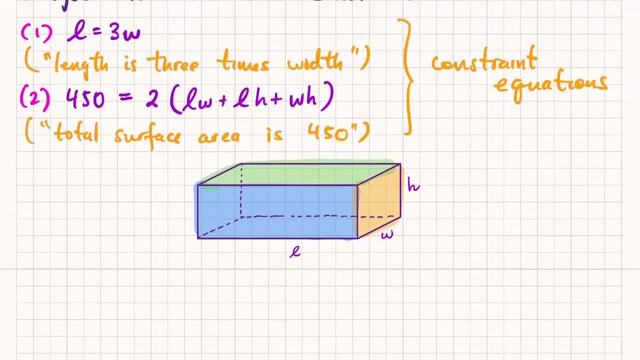 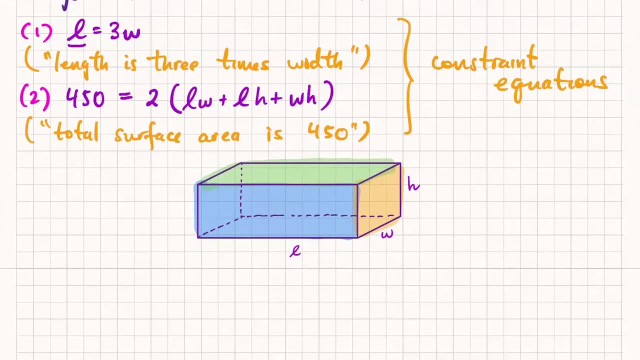 Put a constraint in terms of one variable. OK, good. So it doesn't matter what variable you choose, but I think L is already in terms of W, So let's just put everything in terms of W. That'll make everything a little bit easier. 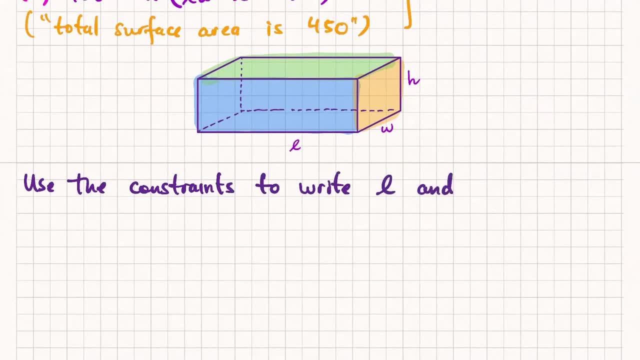 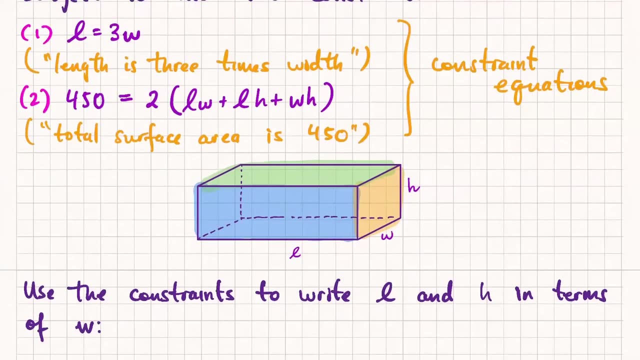 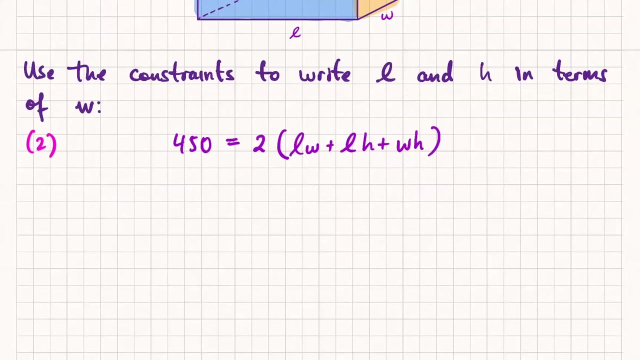 Use the constraints to write L and H in terms of W. So, looking back at this surface area, I made those constraints, So I put in what? So first of all, 225.. I'm just going to divide both sides by 2.. 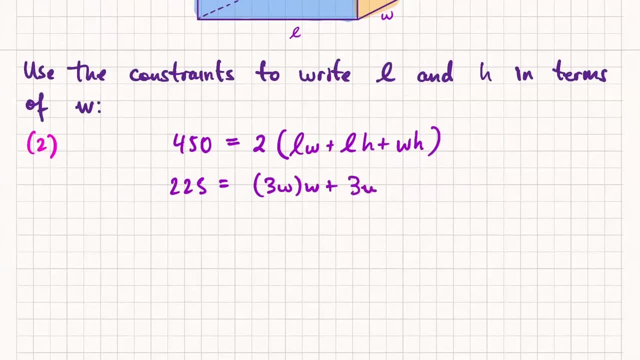 The L is 3w, So I have 225 equals 3w squared plus 4wh. Remember I'm solving for h, So I get what h equals 225 minus 3w squared, So I put in 225.. 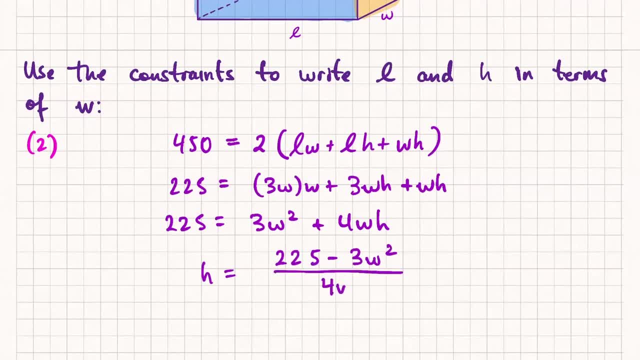 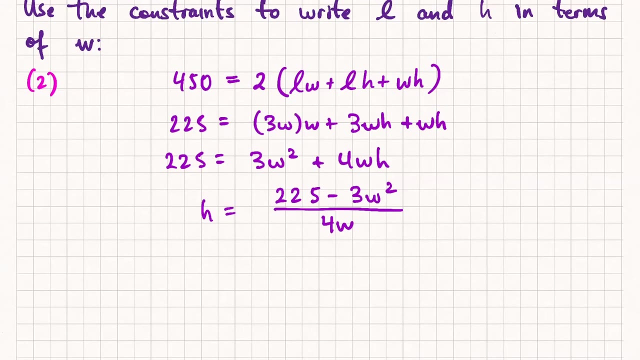 I'm just going to divide both sides by two minus 3w, squared all over 4w, and so that's my equation for h in terms of w. just very simple algebra, right? okay? so i have l in terms of w, i have h in terms of w, and now let me go back to 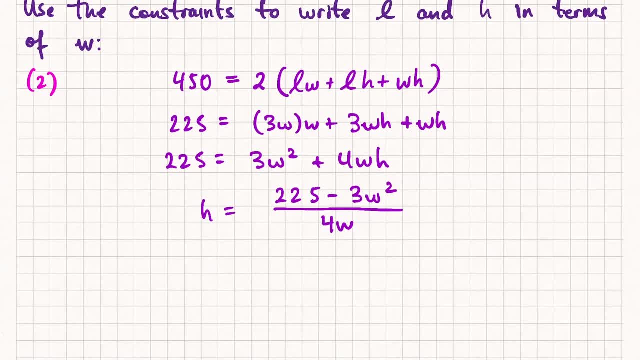 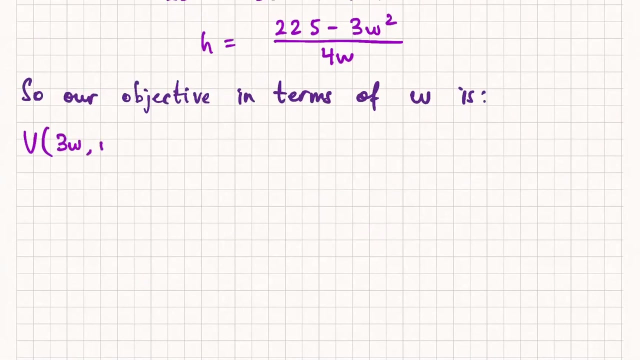 my original constraint to get everything in terms- not my original constraint, sorry, my original objective function and get everything in terms of a uh w, right, because right now my objective is lwh. i want that only in terms of w, so our objective in terms of w is okay. so my volume was l, so l is 3w and h is 225 minus 3w squared. 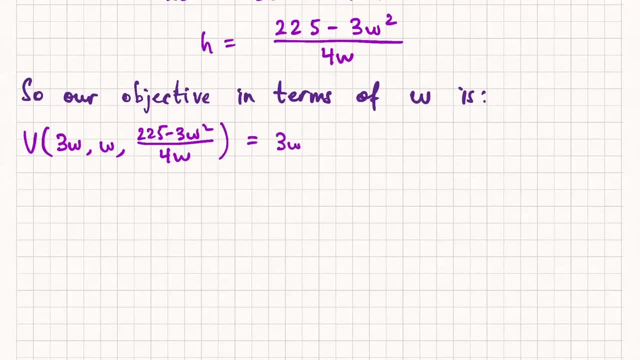 over 4w. so if we multiply these three things together, let's see a little bit of algebra. this should simplify, because i think we get some stuff that cancels out right. so let's see a w cancels out, and then i can maybe distribute the w. 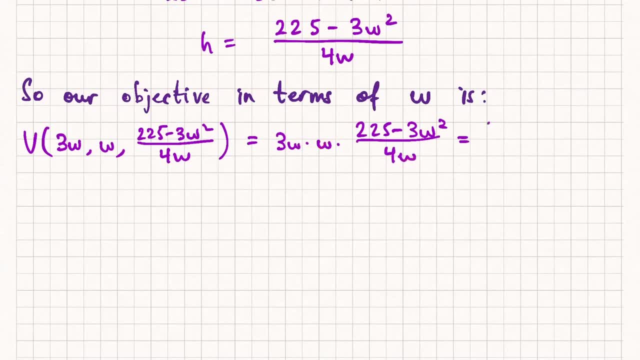 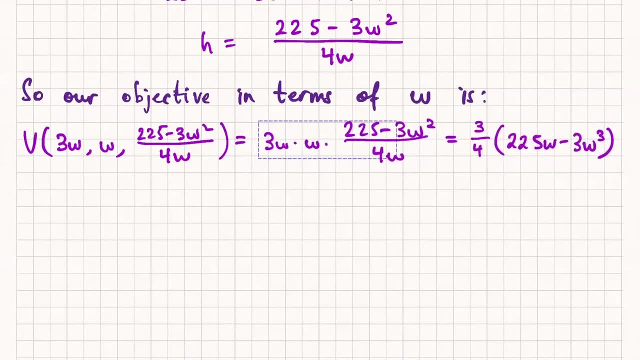 okay. so again, that's just a little bit of algebra, so make sure you actually cancel all that out yourself. now let's talk about the interval of interest. any questions so far about identifying the constraint, the objective, doing all this algebra? so far we have not done any. 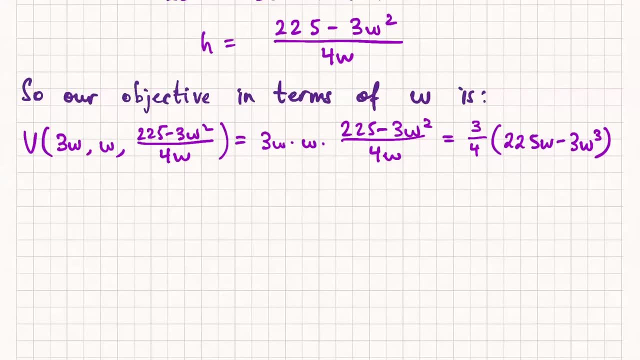 calculus. i want to make that clear. if you have any questions, feel free to email me at the internetcom. that clear. So far no calculus has been done. Any questions so far about any part of the problem. This is more difficult because there are three variables right. It is a little bit trickier to. 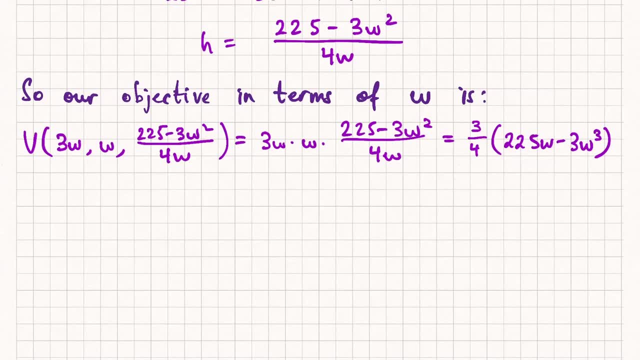 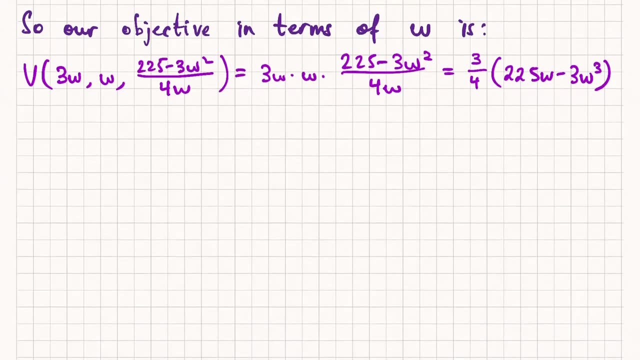 set up. Margaret, what about you? Do you have any questions? No, No, you're good. Okay, Let's talk about the interval of interest. Okay, this is actually pretty tough for this problem, So I'm going to kind of explain it to you guys, instead of asking for it. 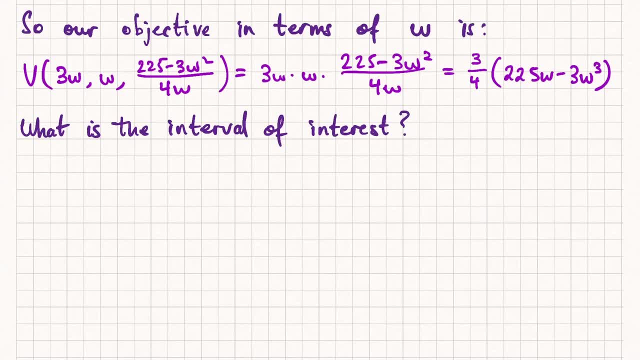 So, first of all, I'm going to talk about the interval of interest. So let's talk about the first one. So let's talk about the interval of interest. So let's talk about the interval of interest. So of all, in general, when you have lengths, a lot of you have so far realized that lengths have to. 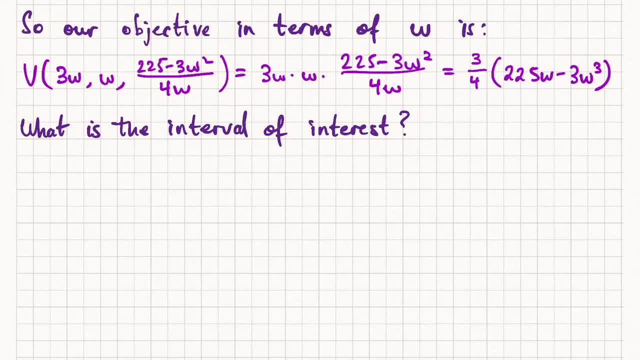 be positive. Actually, lengths don't have to be positive. They can be zero. So lengths are allowed to be zero. We call these degenerate cases. So, for instance, if I have a rectangle, so here's L and here's W for a rectangle, If I have, L equals zero. what does a rectangle with length zero look? 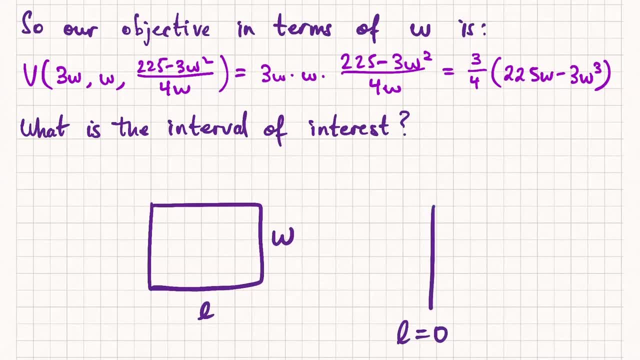 like It's literally a line segment, right? So if you're talking about, say, the area of this, right, the area of this might be, say like 10 or something. What is the area of this? The area is: 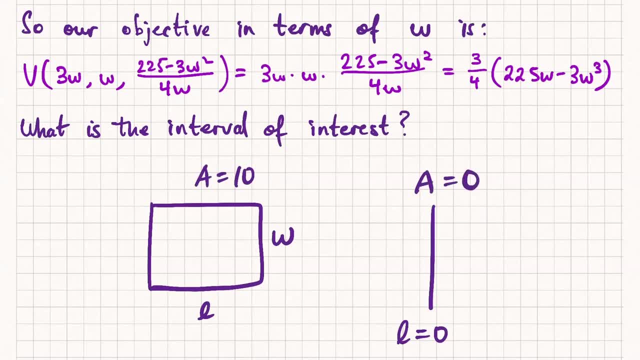 zero, The reason why I actually want to math. it might seem weird to include L equals zero as a case. I mean, why would you want? why would you consider length equals zero? There's actually a good mathematical reason for it. If you're allowed to include the endpoints, right, that's actually. 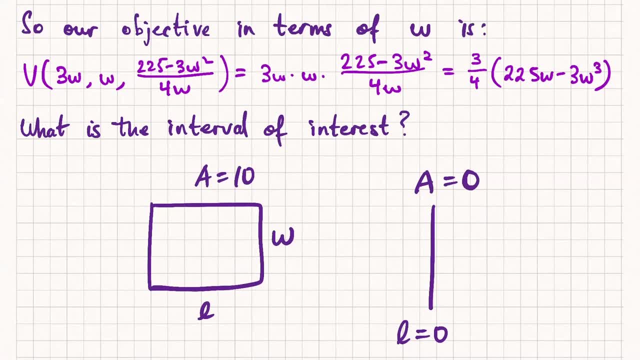 better for us because we know from 4.1, if the endpoints of the domain are allowed to be included in consideration, then we have a lot easier time finding them in our max right, Because we might be guaranteed them in our max. You can just check the endpoints and 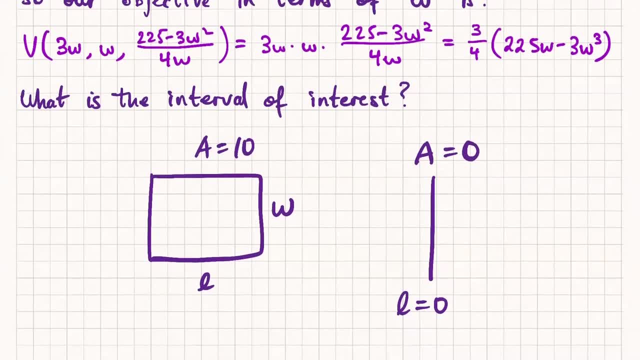 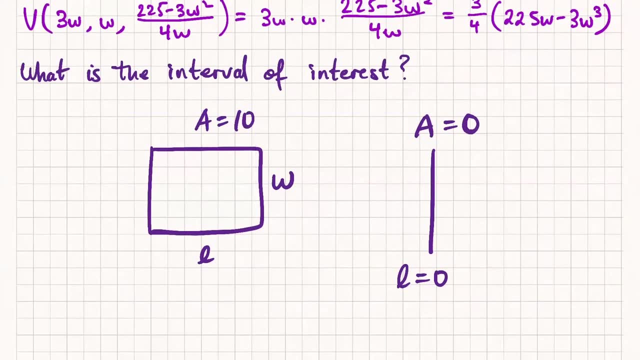 the critical points. right, It's a lot easier for us. So in general, you should include the endpoints if it makes sense. So length equals zero is perfectly okay. So, having said that, that means in our problem we must have that L is greater than or equal to zero, W is greater than or equal. 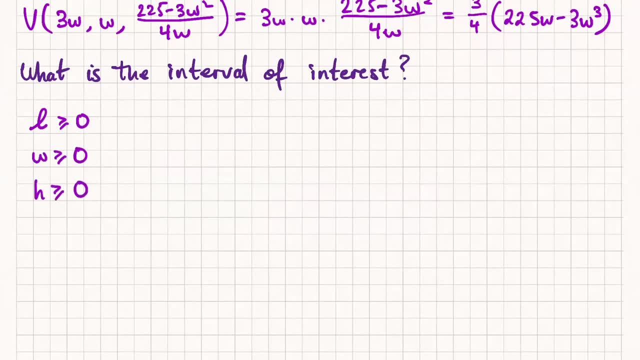 to zero and H is greater than or equal to zero. But what does that mean? It means that we have L equals zero. What does that mean in terms of W? Well, in this particular case, L being greater than or equal to zero just means 3W is greater than or equal to zero, which is the same thing. 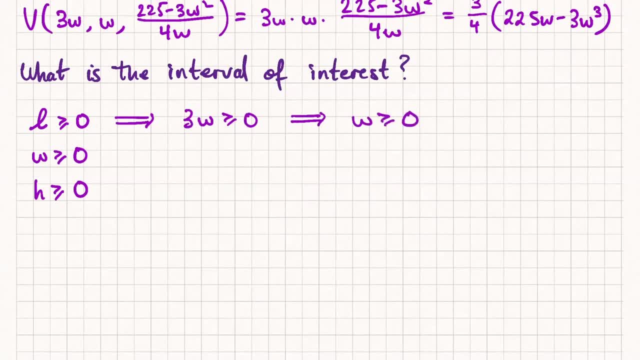 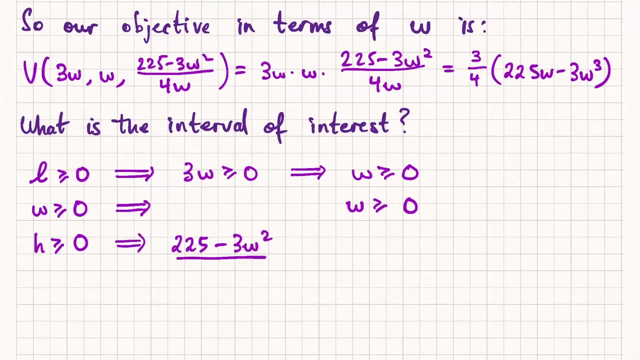 as W is greater than or equal to zero, Remember, because L is just 3W, So that doesn't really affect anything. The W doesn't really give you anything either, But the H, however, actually does give you something. This was the expression for H in terms of W. 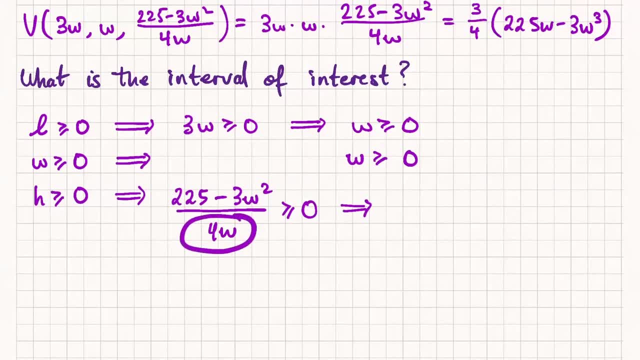 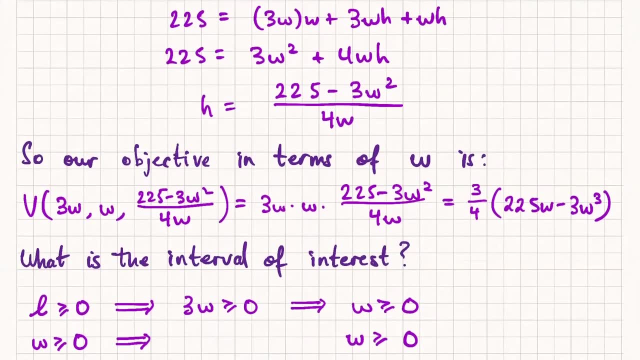 And this actually tells you a few things. So first of all, if I'm dividing by W, W cannot equal zero. Otherwise H is not even defined right. That makes sense because if you go back to the constraint equation for surface area, W equals zero would give you 225 equals. 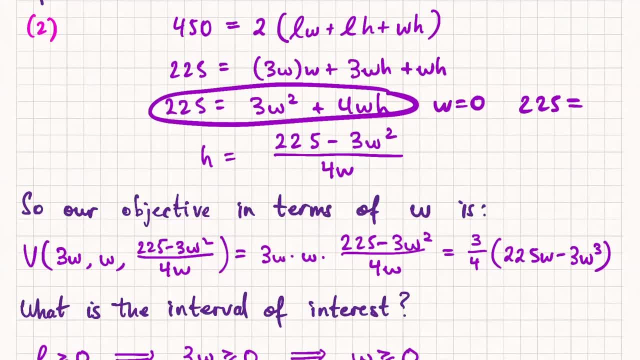 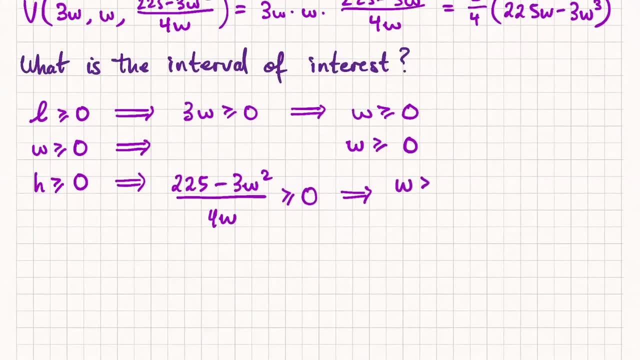 zero. That makes no sense. So W actually cannot equal zero in this particular problem. But in general you might allow lengths to be zero. So W actually has to be not equal to zero. And then if you solve the numerator greater than or equal to zero, 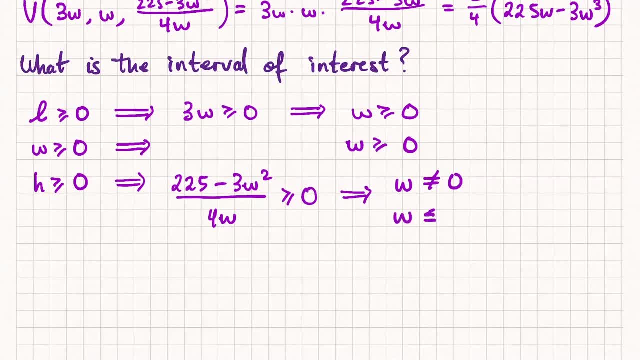 you just get what W has to be less than or equal to square root of 75, right? And that 75 is coming from square root of 225 divided by 3. So that's square root of 75. So this is actually a very interesting problem to get the interval of interest. 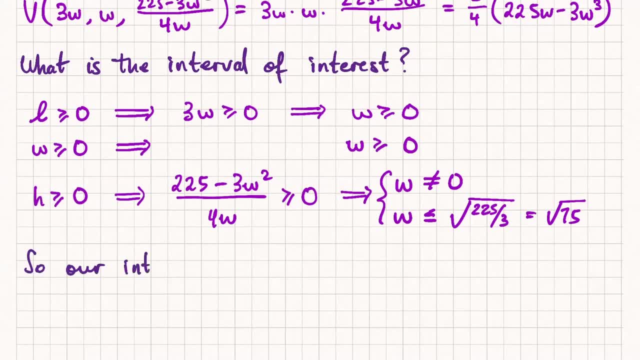 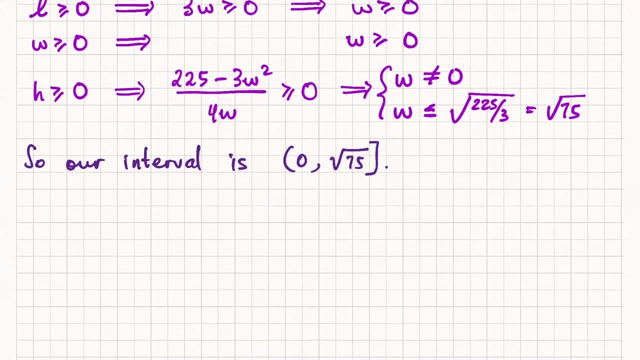 So our interval is curiously zero to square root 75.. The zero is not included, but the square root 75 is included. That's interesting. You might want to later think about what it would mean for W if W goes to zero. you actually get a box that's literally just a stick. 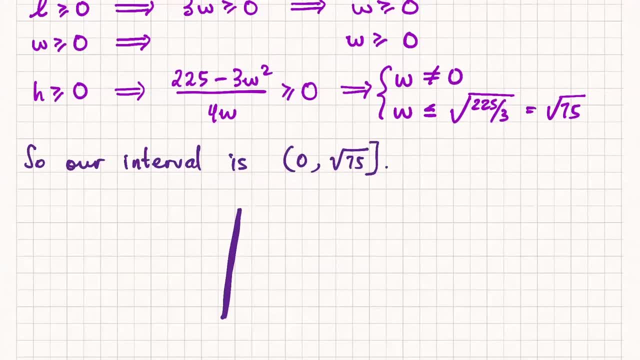 So no surface area. But the square root of 75 gives you a box that's literally just like the lid. So there is surface area. So it's interesting to think about what the extreme cases actually correspond to. Margaret, you're confused. You have a scrunched up face right now. 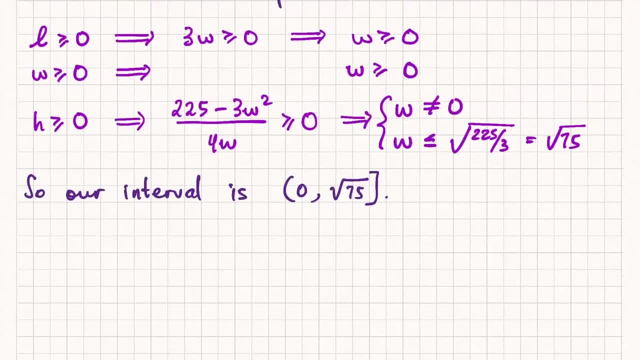 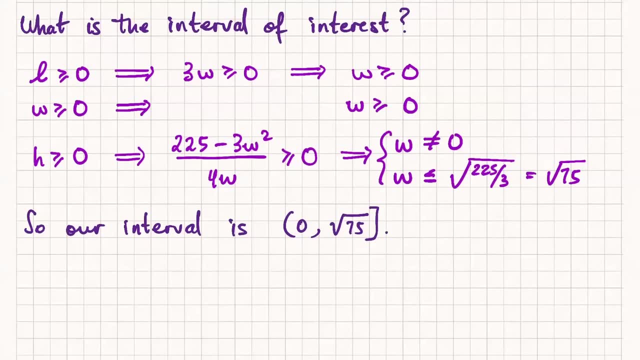 What's your question? I don't really have a question, but I didn't really get it, So get what Which question? So you do have a question Like the H, like the interval, Well, the H interval. So just to very quickly go over that, 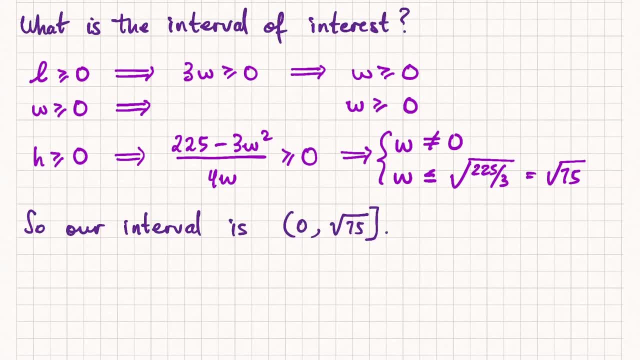 I'll take notes to think later. No, we can think now also, Caleb. So just to make very clear: So this was the expression for H And if I'm saying that H has to be non-negative, right Length has to be non-negative For this thing to be non-negative. 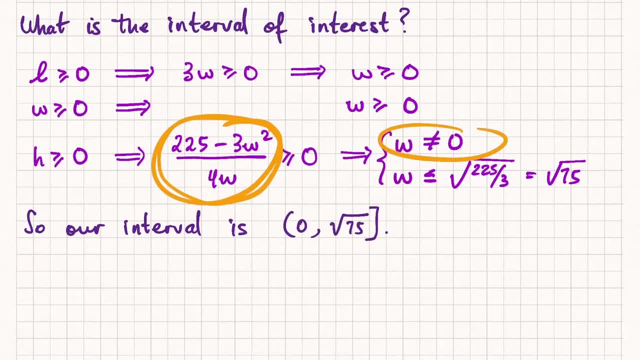 first of all, you can't divide by zero, So W can't be zero, So that's why zero is no longer included. The second thing is, if you set this greater than or equal to zero, well, remember, W is positive. 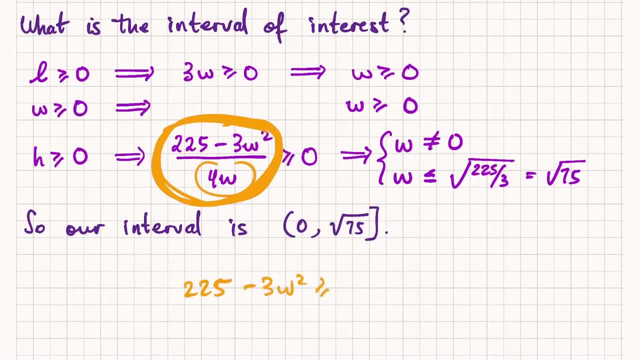 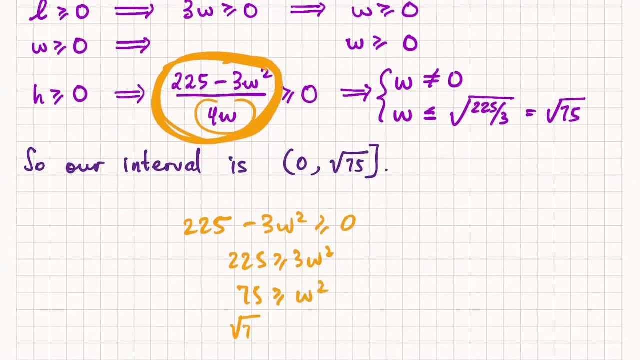 So you get 225 minus 3W, squared greater than or equal to zero. And then this is just some algebra right, Divided by 3, 75 greater than or equal to, and then take a square root. Okay, So that's how we get that. 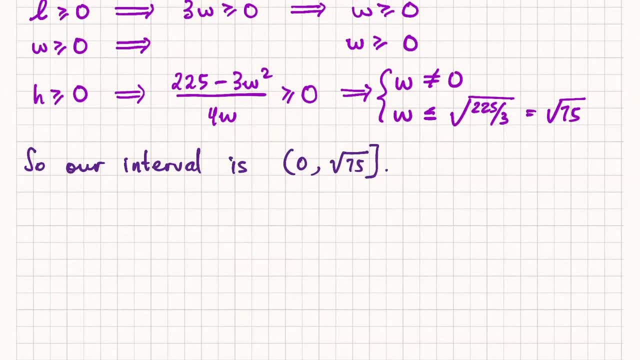 The nice thing is W is positive, So you don't have to worry about, like, switching the sign of anything. In any event, let's write down our goal. So our goal is to find the dimensions of the box right, So find the value of W. 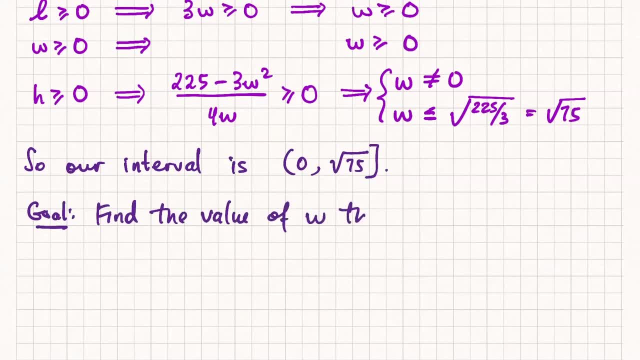 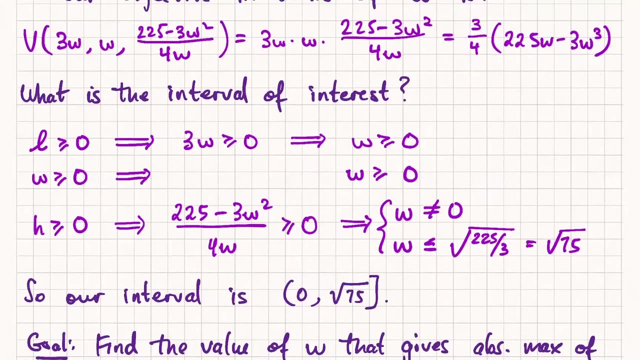 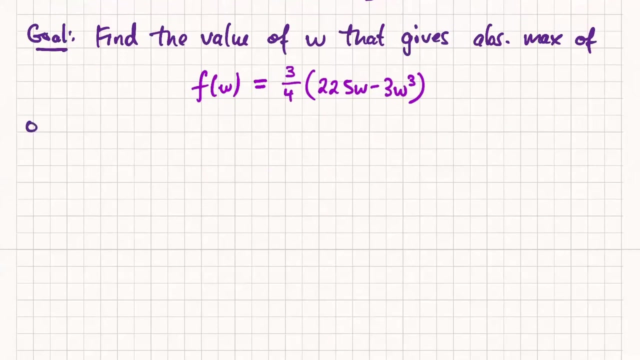 that gives the largest volume. right, That gives absolute maximum of my function, And we've almost forgotten about that. what the function was. The function was this thing up here: the volume: Okay, On the integral 0 square root, 75.. 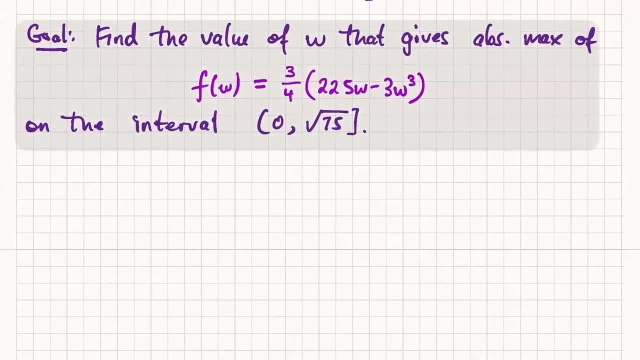 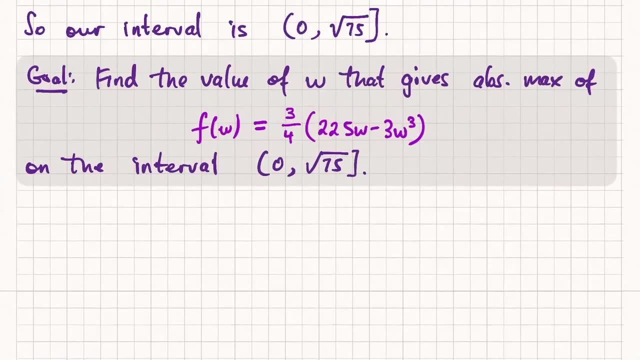 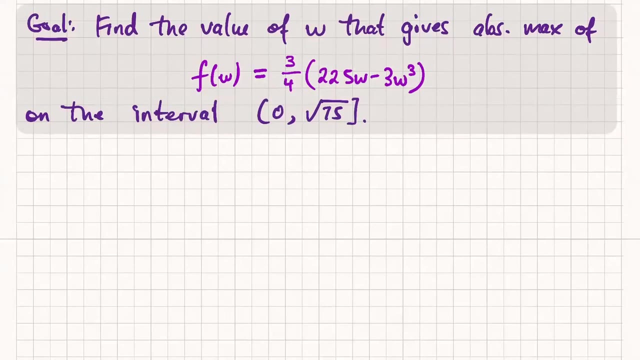 Now what's going to be really fun about this problem is the interval is actually not going to matter anyway. So all of that was for naught, But we have to actually kind of see exactly why the interval is not going to matter. Any questions up until this point. Again, this is the non-calculus. 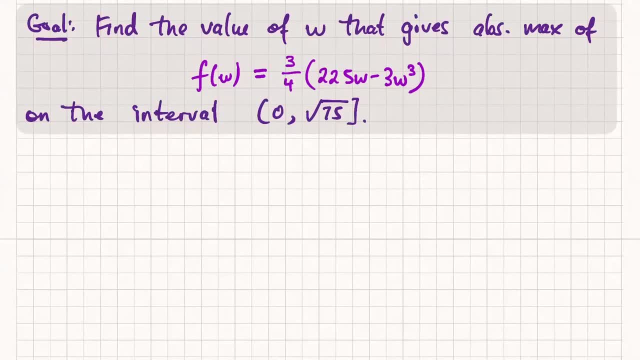 portion of the problem. So if you have any questions, please feel free to ask them in the chat. We have nothing, any calculus, no limits. no, nothing right, No limits, no derivatives, nothing. A lot of students usually find the first part of the problem sometimes the hardest part of the 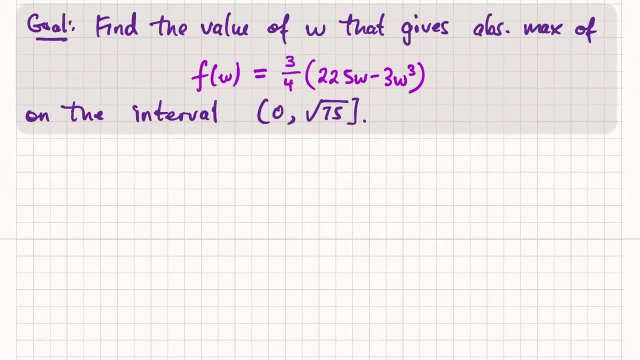 problem And I, you know it's. it's sometimes not easy, Okay, So now the last part of the problem is: you know, find the critical numbers, Then we do our justification. So we may not finish this in the next two minutes, but that's fine, We'll finish. 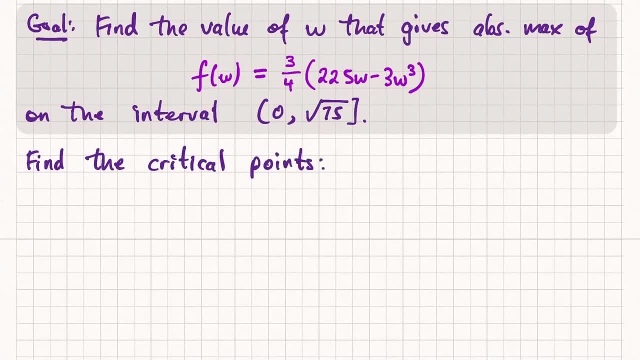 up on Tuesday. So my derivative is 225 minus 9w squared. Set that equal to zero And you get w equals 5.. You actually get plus or minus 5, but the minus we don't, we don't care about, right. 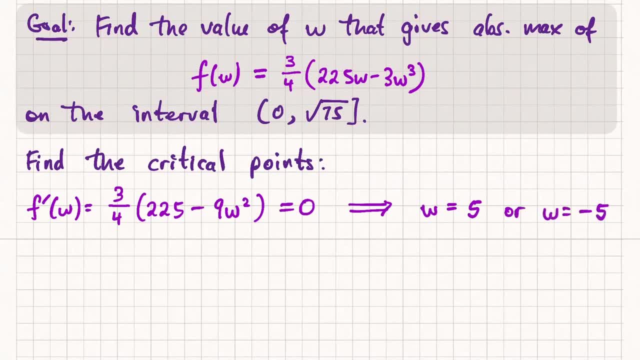 Maybe I'll actually write that Right. We don't care about the minus 5.. You get the minus because, remember, you're taking a square root with the w, So that's why you get two values of w. Do you actually get 5?? I think you should get 5.. 225 divided by 9 is 25 squared. 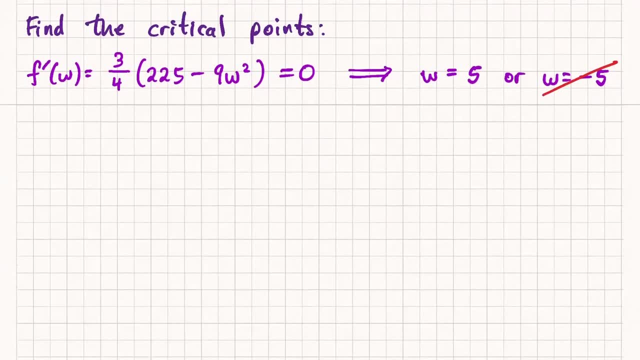 is 5.. Okay, good, Okay, So now you have a few things at your disposal, right? You've pretty much solved the problem. You've pretty much found that w equals 5 will give you the largest volume, hopefully, but you do have to justify it right. In the last two examples, we've always justified 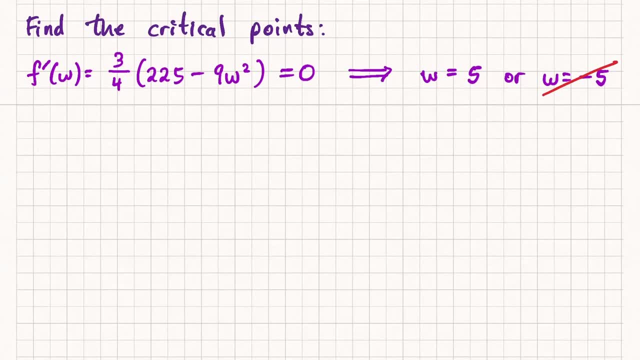 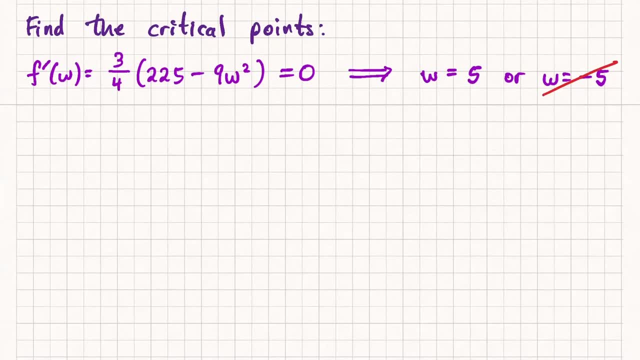 derivative test So you can use either or You don't have to use both. Use either, or They gave you the same conclusion. Now, typically for me I usually go the second derivative test route, because I just think usually finding the second derivative isn't too bad, If finding the second. 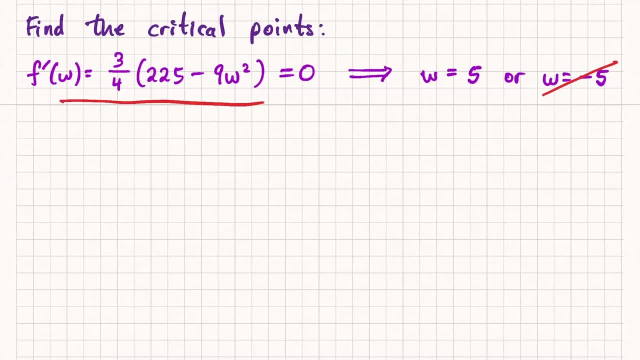 derivative is kind of going to be a nightmare. then just do the first derivative test, But for me I think the second derivative in this case is pretty easy. So observe that the second derivative is 3 fourths times negative: 18 w, And that's obviously negative. if w is positive, which is 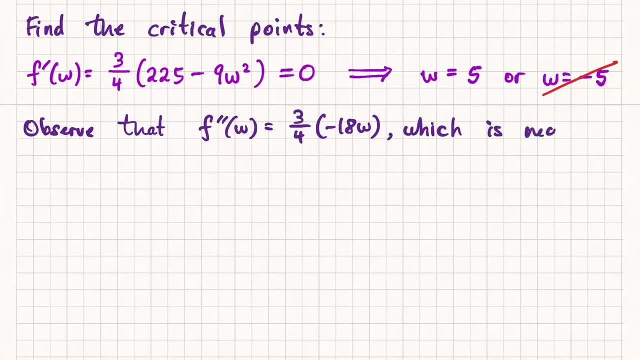 negative for all w greater than zero. And what do we know about negative? If I have a negative second derivative in the last minute of class, Rachel? a negative second derivative means what about the concavity? Yeah, concave down. And if I have concave down, that means whatever critical point I found.